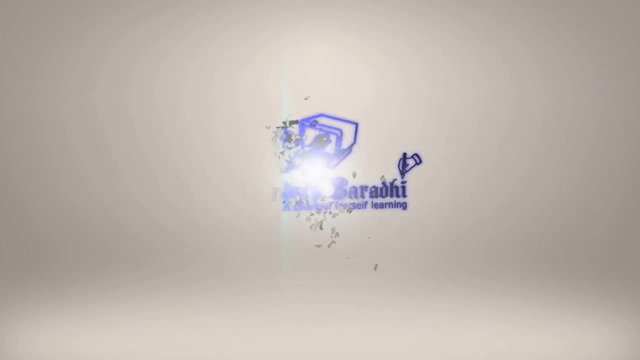 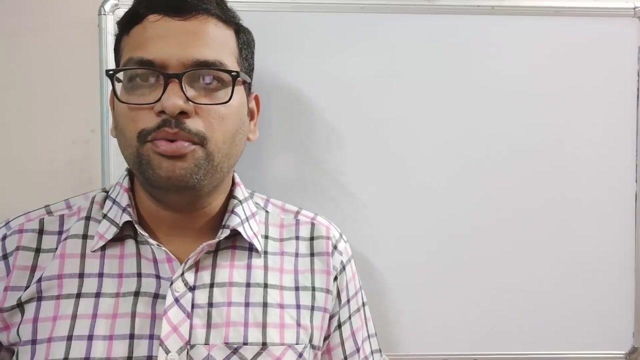 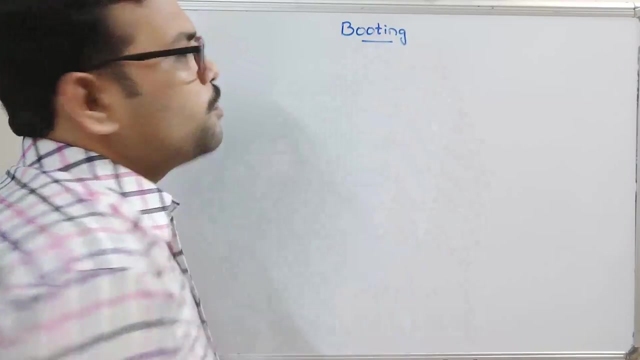 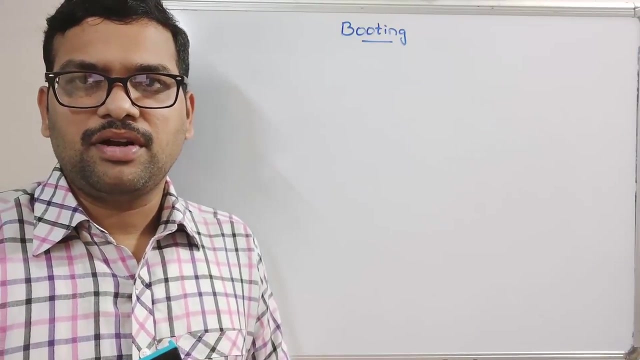 Hello friends, welcome back to our channel. So in today's session we will discuss about the process of booting. So what is this booting process? So in the previous session we have seen how to create the bootable drive and how to install the operating system in our hard disk. 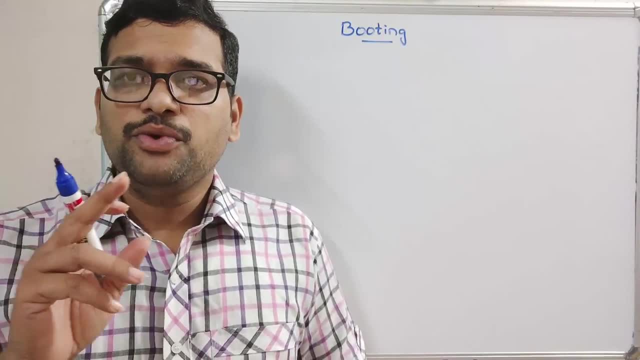 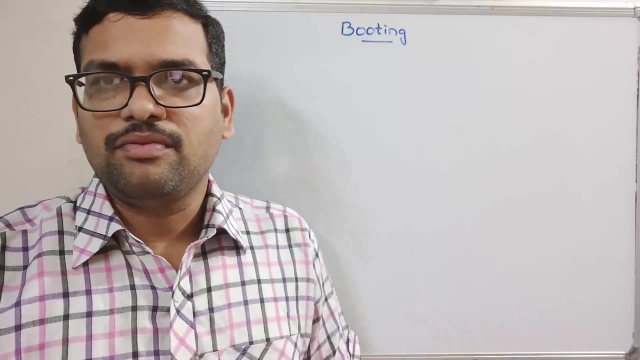 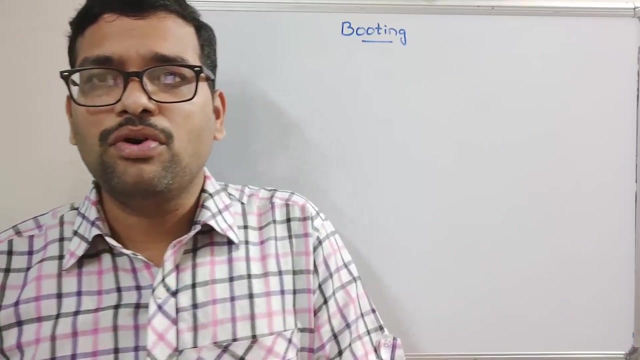 And in today's session we will see about this booting. So whenever the user presses the power button, automatically the operating system will be loaded and the user will start working on the computer. So whatever the process that has been done after pressing the button and before loading the operating system- is called the booting. 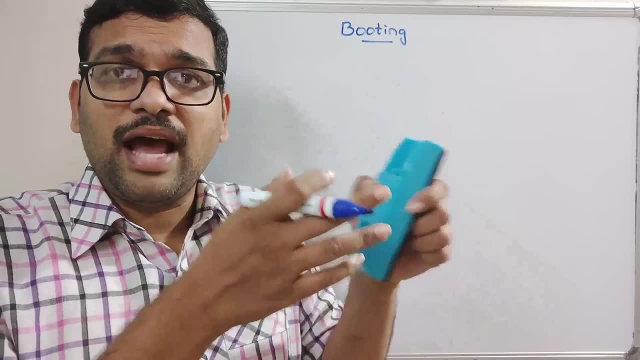 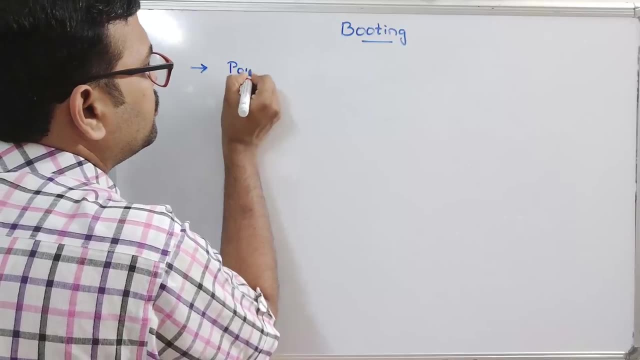 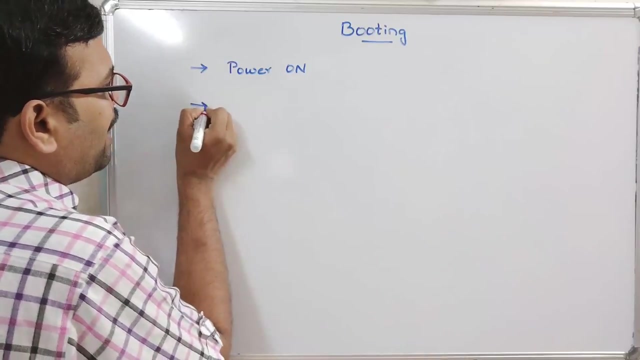 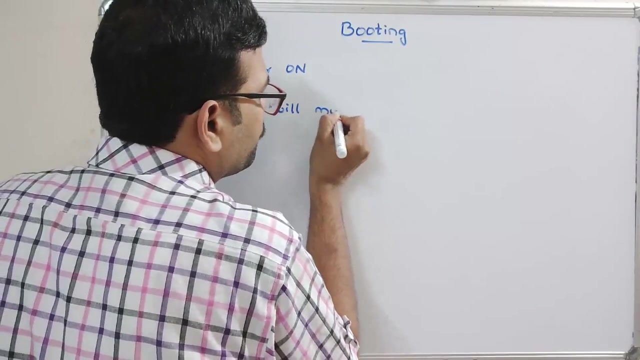 So we will see what are the steps Or what are the things that happens during this process. So the first step is power on, So the user clicks on the power button. So immediately after the user clicks on the power button, the CPU will move to BIOS, which is available in ROM. 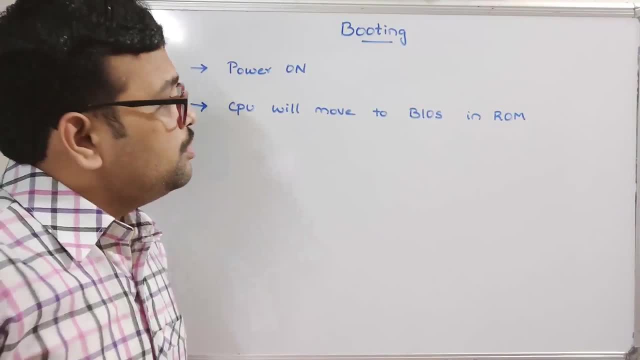 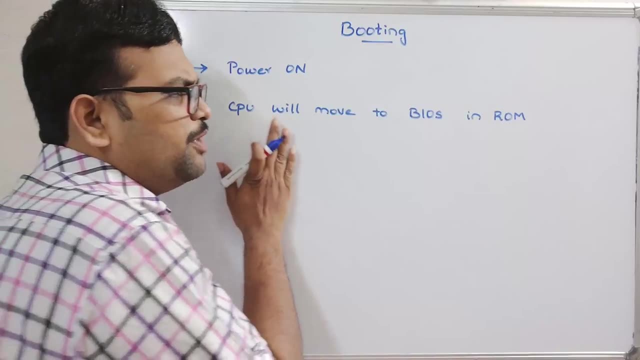 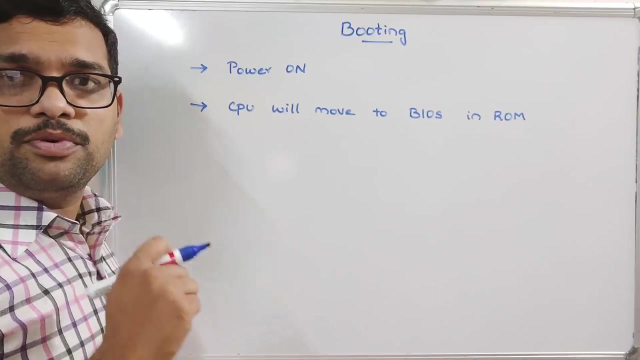 So ROM is read only memory. So immediately whenever the user clicks on this power button, press this power button automatically, the CPU will first move to the BIOS in ROM. What is the BIOS? BIOS is a basic input output system. Basic input output system. 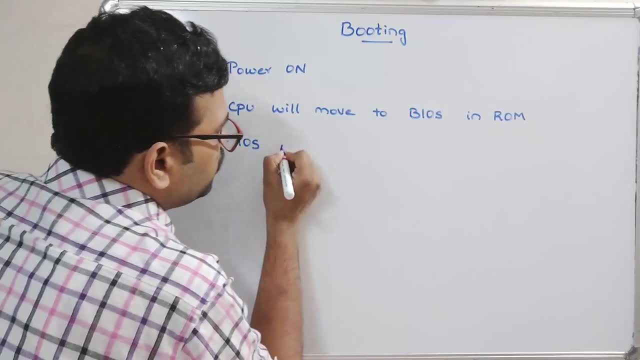 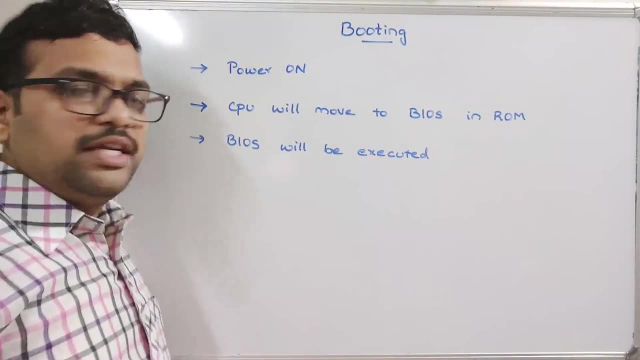 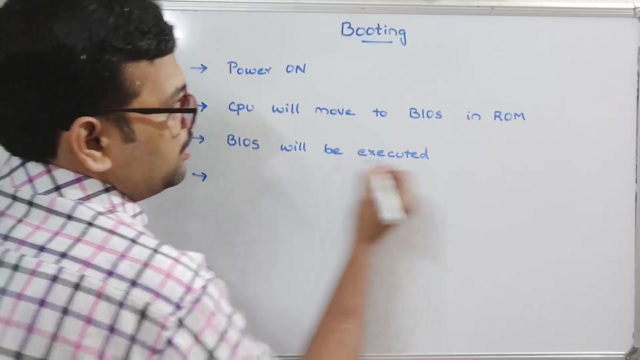 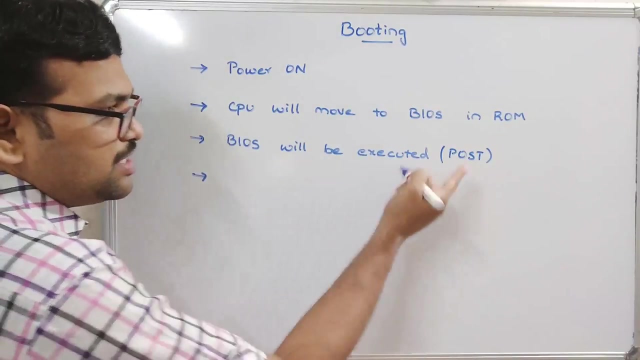 And the next step, BIOS, will be started. execution- BIOS will be executed. So what actually will be executed by the BIOS? So it will be done: the POST, The POST, will be done. So what is this POST? POST means power on self test. 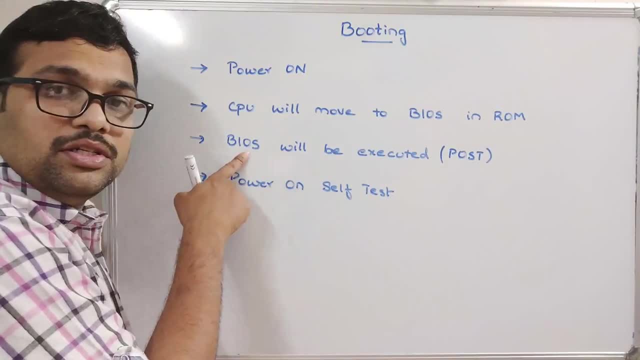 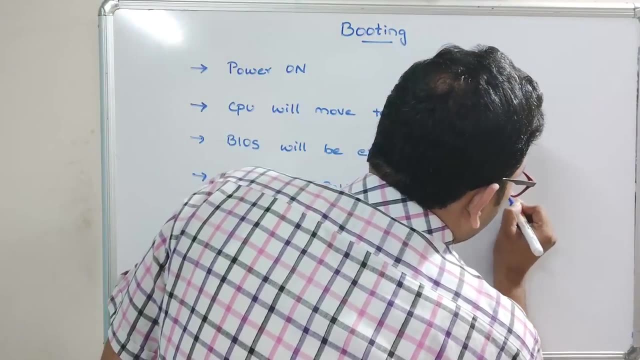 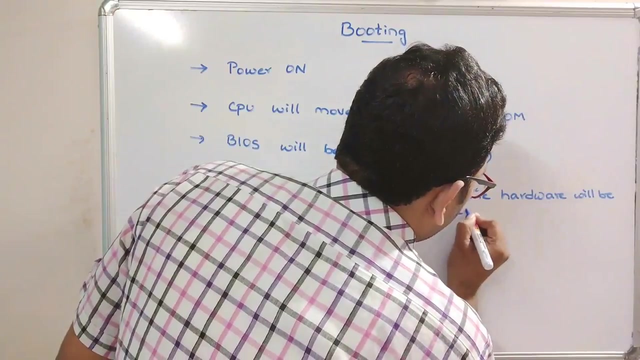 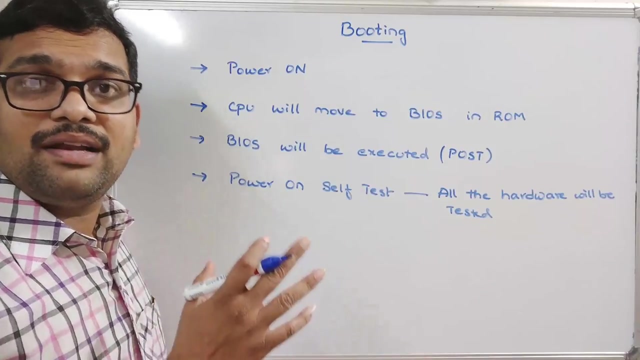 So this process will be executed by the BIOS. So power on self test. So here, all the hardware will be checked. All the hardware will be tested. So whether the hardware related to this CPU are working condition or not, If the hardware is not working condition, automatically the booting process will stop. 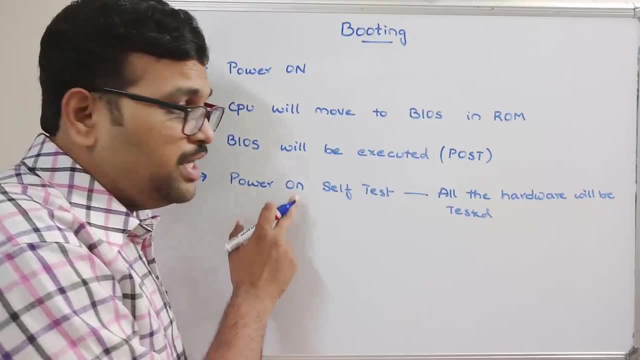 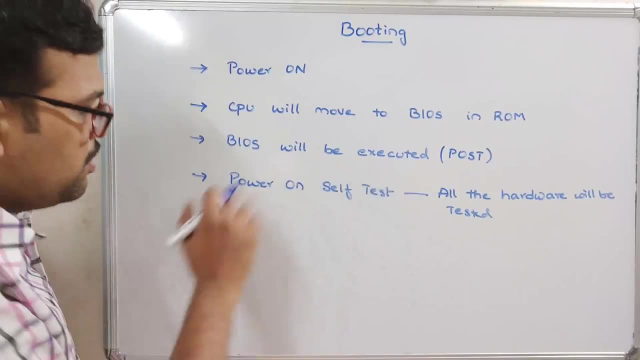 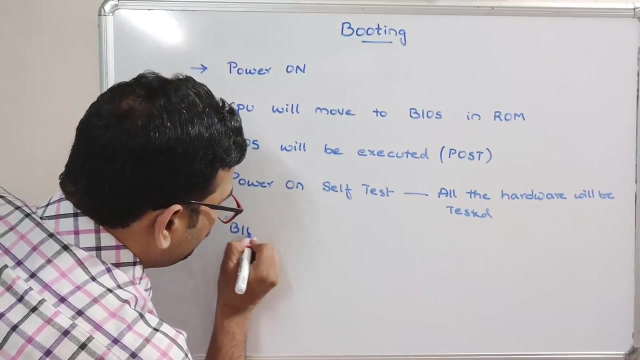 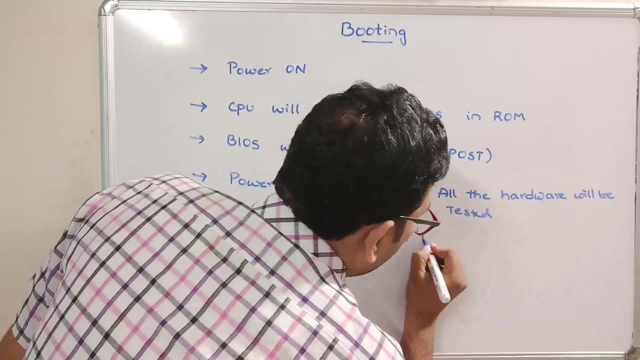 So if this POST is successful, If this POST is successful means so the hardware is working condition. So whatever the hardware related to this CPU will be in a working condition. So now, after that, immediately, whenever the power on self test is successful, immediately the BIOS will load NBR to RAM. 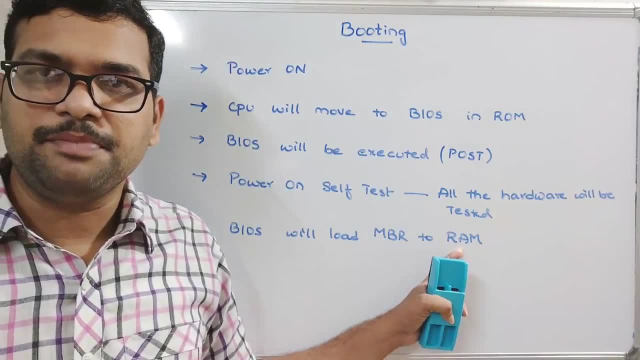 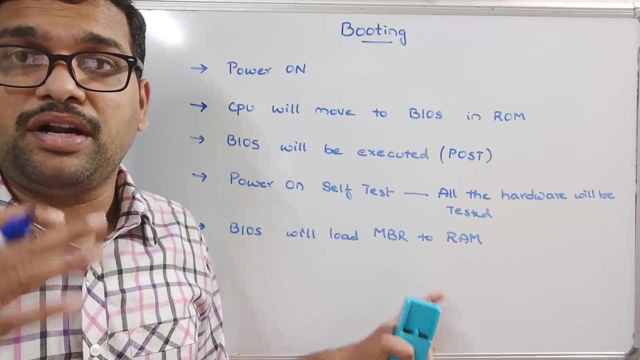 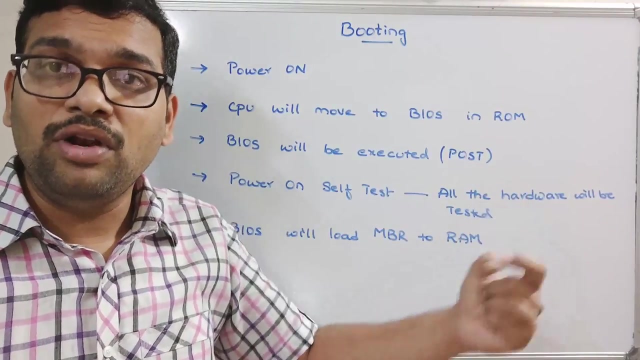 Now there is one more term called RAM, Random Exist Memory. So the NBR, it will load the NBR to RAM. NBR means Master Boot Record, Master Boot Record. So previously we are checking only the hardware. So after the hardware is working condition, then only we need to load the software into the RAM. 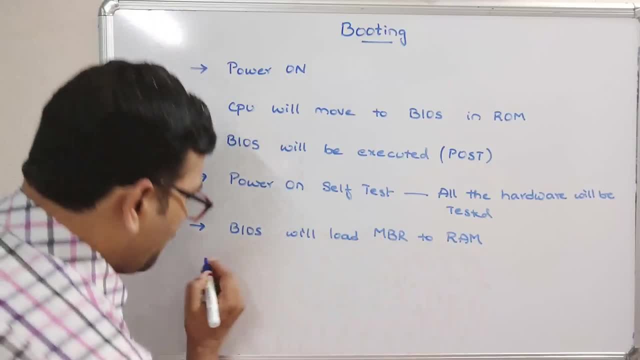 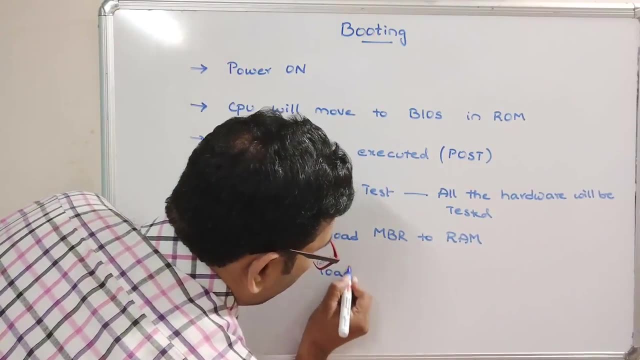 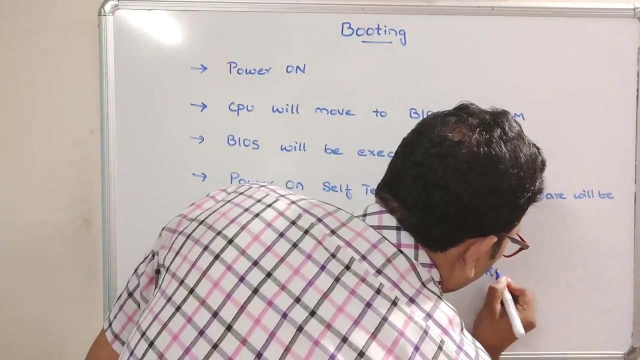 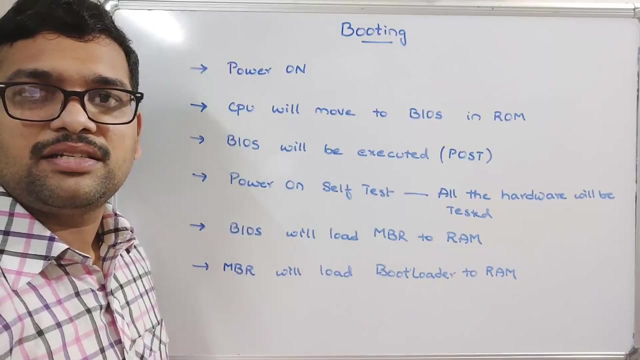 So NBR is a master boot record that will be loaded into the RAM. Now the NBR- NBR will load boot loader, Boot loader to RAM. So what is this boot loader? This boot loader is the thing which loads the operating system to the RAM. 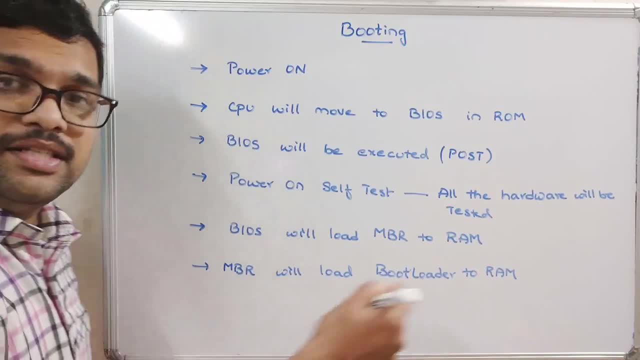 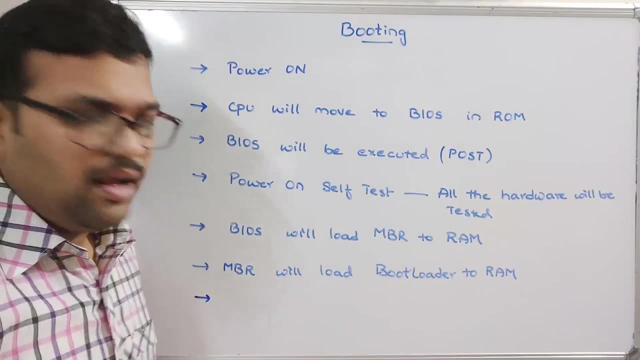 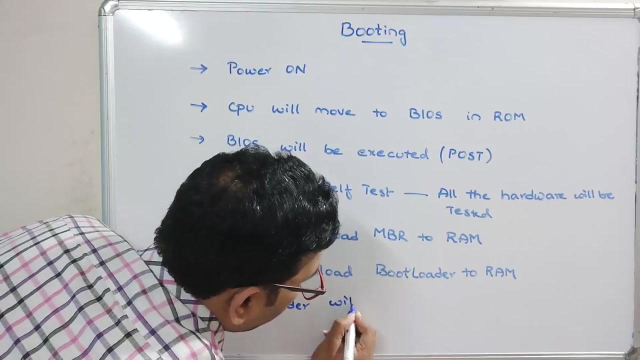 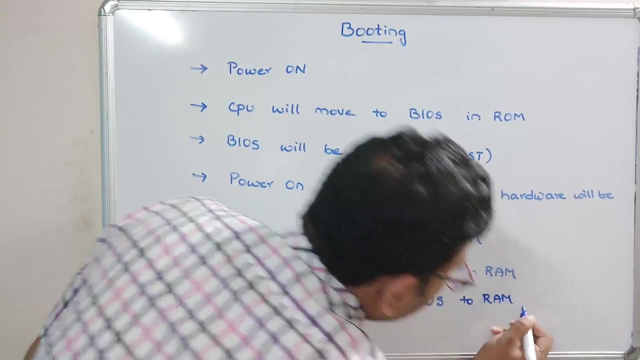 So this boot loader will load the operating system into the RAM. So here there are different stages of boot loader, So stage 1 and stage 2 will be there. So now this boot loader will load operating system to RAM and it starts executing the operating system. 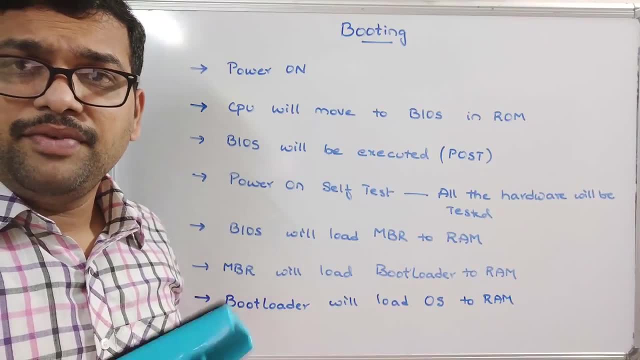 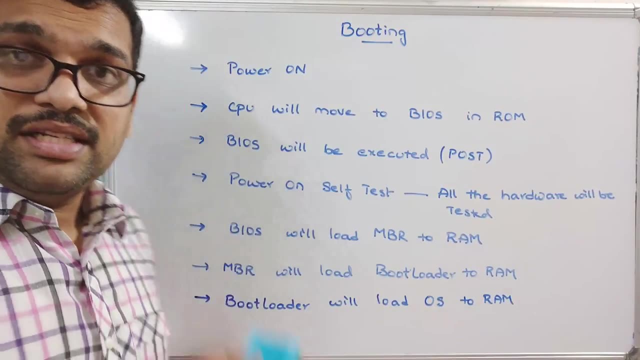 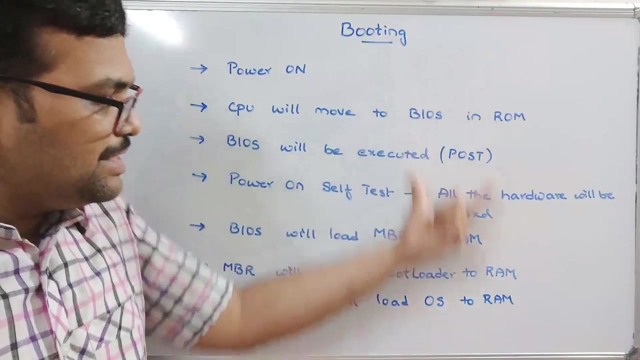 So, whatever the operating system- it may be the Windows or Linux- it will load the operating system into RAM and automatically the control will move to the operating system. So this is what happens during this booting process, That means whenever the user power on the system. so all this happens and finally the control will be moved to the operating system. 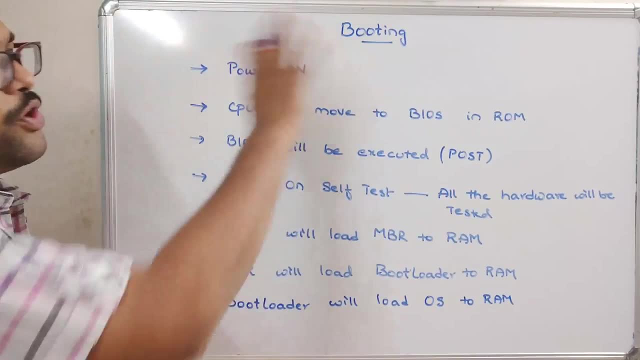 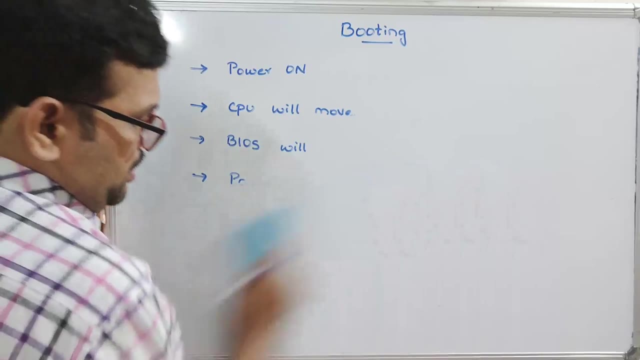 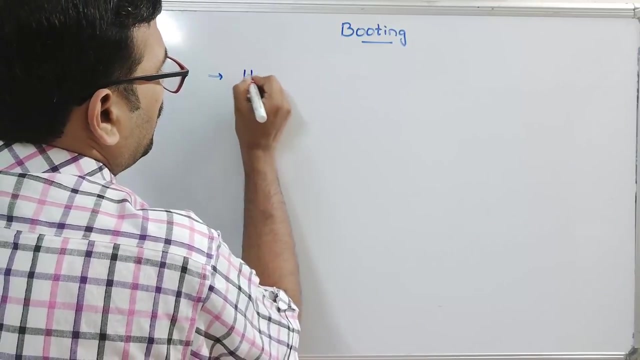 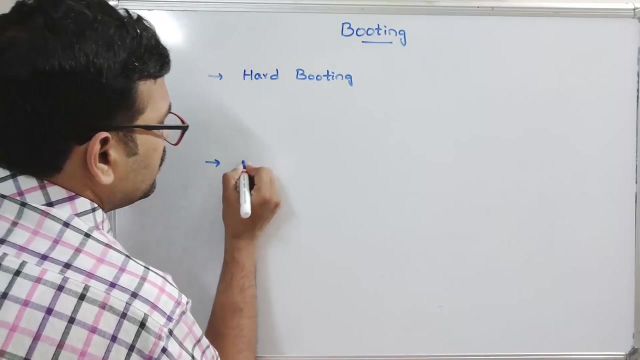 So this is the process and this process we call as a booting. So there are different kinds of booting. So there are different kinds of booting. See whenever. the first type of booting is hard booting and soft booting. So there are two types of booting process.